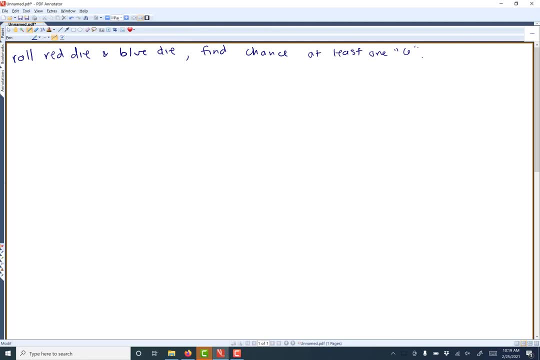 So if I was going to roll these two dies- and I want to find the chance of at least one six- when we do probability, the biggest thing that we need to remember is list out what are all the possible outcomes that will give you what you want. 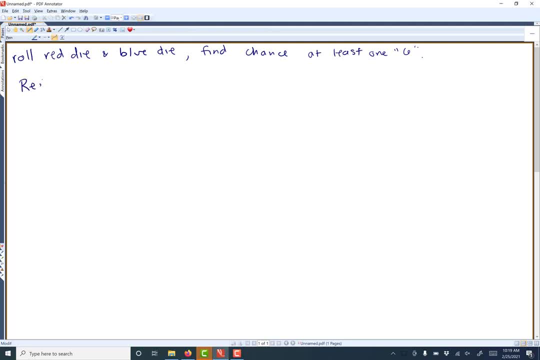 So if you want at least one six, we could do like the red is a six and the blue is a not six. That would be one outcome We could do. let's see red as a not six and we could have the blue as a six, because either of those would have one six. 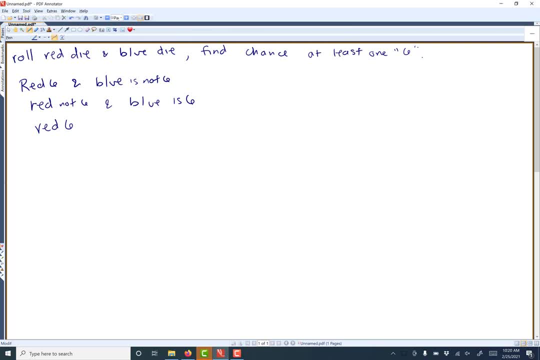 We could also do a red a six, and blue Red is six. Now, on these, when I say, like red is not six, that means it could be a one through five. I really don't care what it is, just as long as it is not a six. 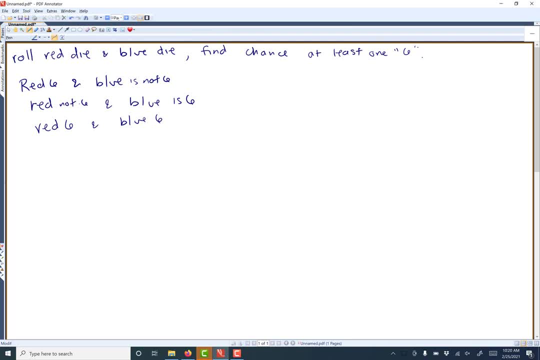 So here are three different possibilities to give me what I want. And if I want to find the probability of at least one six, I'm going to need to find the probability of each of these and then add them up. So, like the probability of red six and blue is not six, 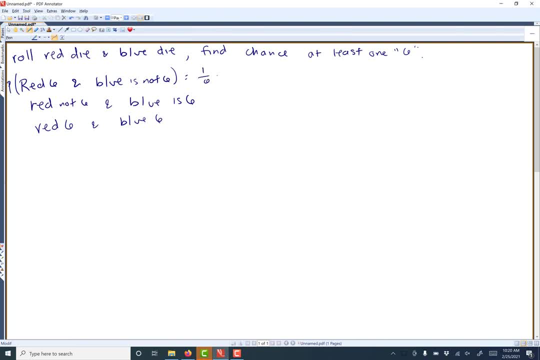 Well, the red six. there's a one in six chance to get a six. and for blue to not be a six, there would be five numbers that are not a six. That's using the complement rule, just in a little step right there. 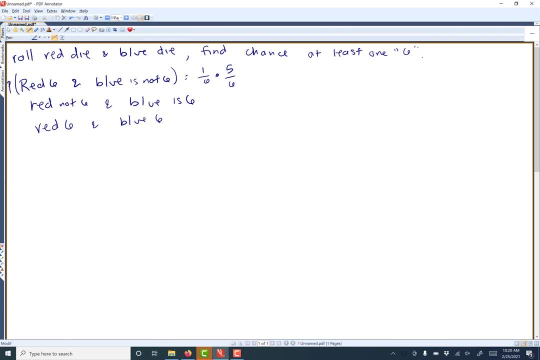 Okay, so if one is a six, that means there's five numbers that are not a six. We're going to multiply because it's an and The two dice should be independent and they shouldn't be affecting each other, so I don't have to worry about that second probability of changing it somehow. 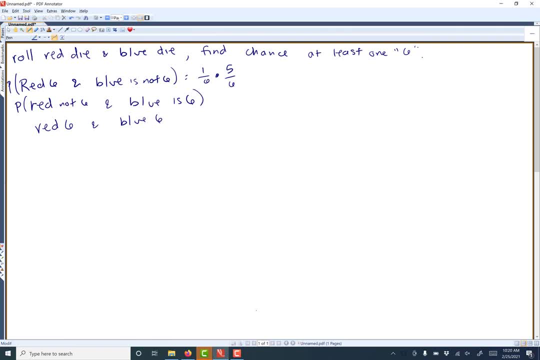 Okay, the probability of the next one for red is not six and blue is six. Well, let's see, we want red to not be six, so that would be five. six times blue is six, That would be one sixth. Now for the last one. if I want red to be six and blue to be six, 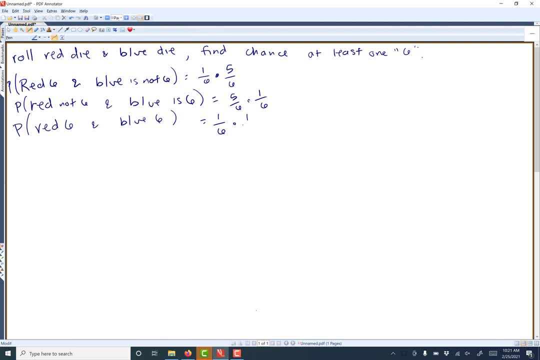 well, we have a one sixth chance of getting red as a six, and for the blue to be six it would also be one sixth. So we would have to find each of those and add them up. So now my final probability. I want to get of at least one sixth. 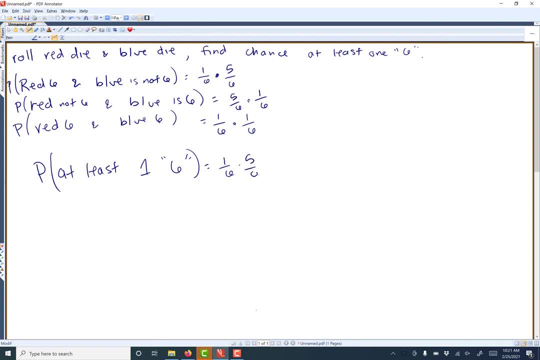 well, that's going to be this: one sixth times five sixths plus five sixths times six, One sixth times one sixth plus one sixth times one sixth, And if I put that in my calculator I should get something like eleven out of thirty-six. 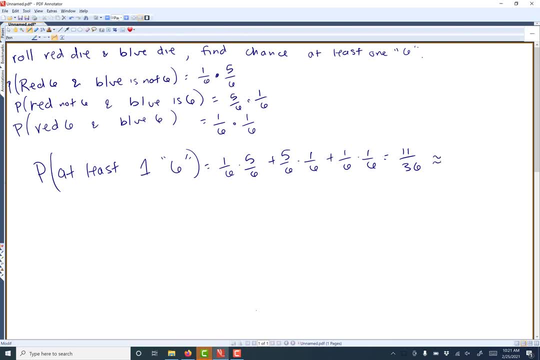 Or if you want to change that into a decimal, because I think decimals are easier to work with point three: oh, five, five. So that's how you can do the probability of at least one the long way. Okay, If it wasn't too long, I only had to find three different probabilities. 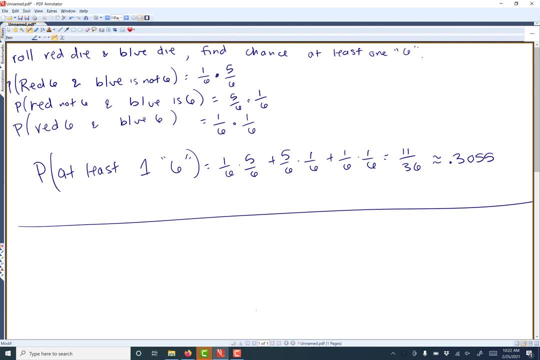 It's really not that hard. But if I rolled even three dice, there's a lot more probabilities that I have to find. And if I wanted to roll six or ten dice, you're never going to finish this problem if you're trying to do it the long way. 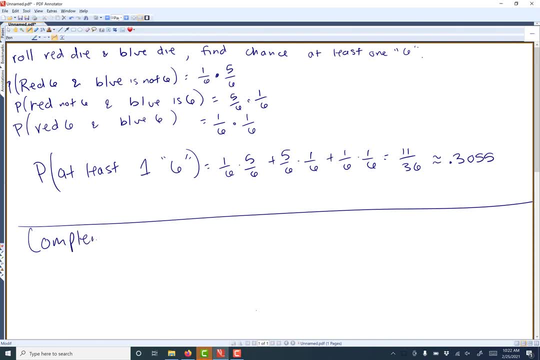 So that's why we invented the complement rule. The complement rule is useful for things like to say: if you have a one sixth chance of rolling a six, then that means you have a five sixth chance of rolling a, not six. So it's useful. 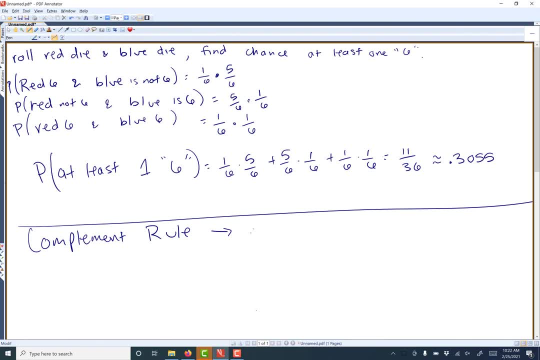 It's useful for nots, but it's also very useful any time you want to find the probability of at least one. We're always going to use this trick for at least one, because it saves us so much time for bigger problems, Because the probability of at least one sixth. 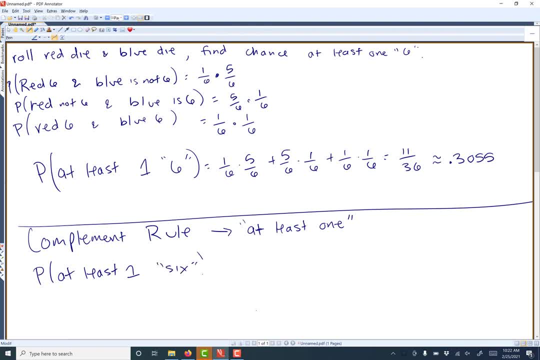 is always going to be equal to one minus the probability of no sixes. Okay, The reason why is, when we looked up these outcomes, those were the outcomes that gave us what we wanted. The only other option left is no sixes. 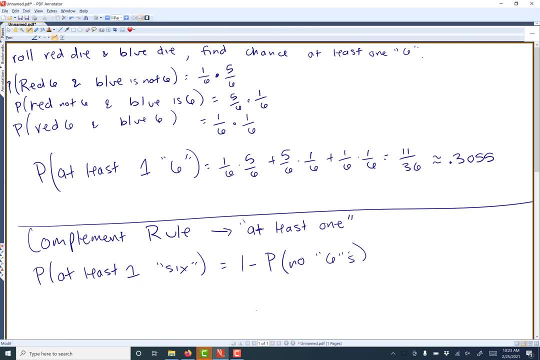 or the complement of at least one sixth is no sixes. So the probability of no sixes, the only way you're going to get that, is if you have red not six and blue not six. So notice, even on this step, when I use the complement rule, 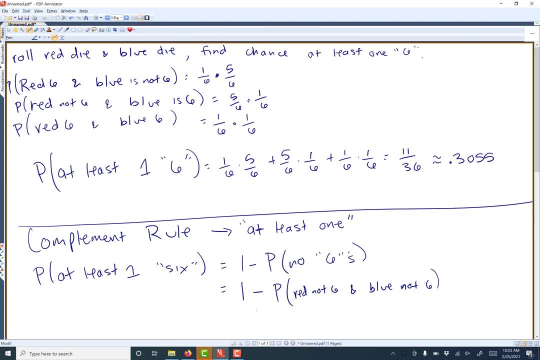 I'm still thinking of, like what outcome gives me what I want or, in this case, with the complement rule, what I kind of didn't want. So the only way to not get at least one is: red is not six and blue is not six.